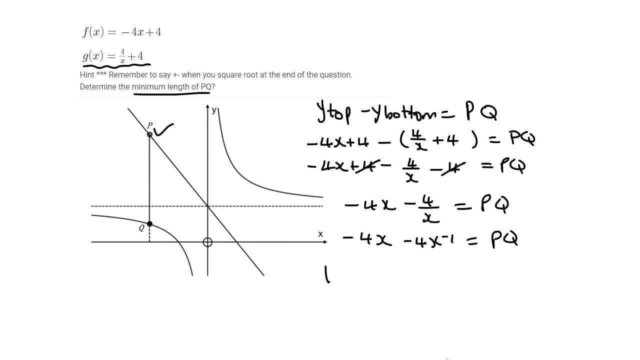 the length of pq. Now we can take the first derivative. I'm actually just going to rewrite this first. just switching everything around just makes it easier. Okay, so we can take the first derivative now, because that's how we find minimums and maximums. That's minus 4, plus because 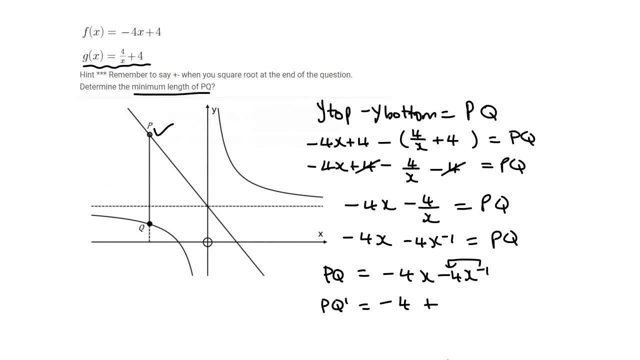 this minus 1 multiplies into the front, and so that's going to be plus 4x to the minus 2. Find minimums and maximums. we make the first derivative equal to 0, like that, and then I'm. 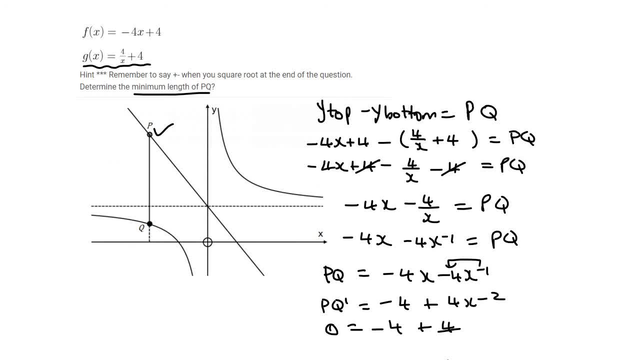 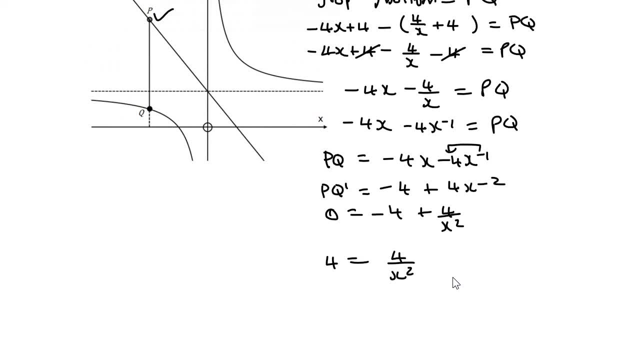 going to put this x at the bottom actually, so it's going to become 4 over x to the 2. Now going to take this 4 over, so it'll look like this: Now we're going to multiply the x squared over. 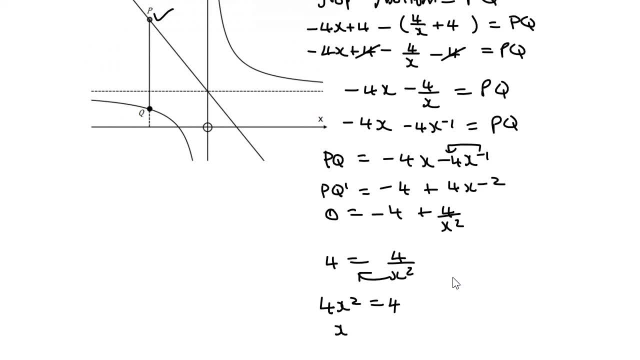 so it's going to be: 4x squared equals to 4.. Divide both sides by 4, so x squared is 1.. Then, when you take the square root, please remember to always say plus and minus 1.. Now they've given us two answers, so we need to now work out which one is the minimum and which. 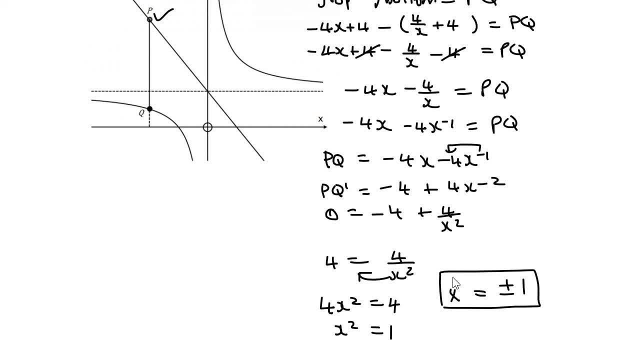 one is the maximum, because when you make the first derivative equal to 0,, that gives you minimum and maximum. Now that we have two answers, we need to check both of them. What is it that we're trying to find the minimum and maximum of? It's the length, and so we made a formula for the length. 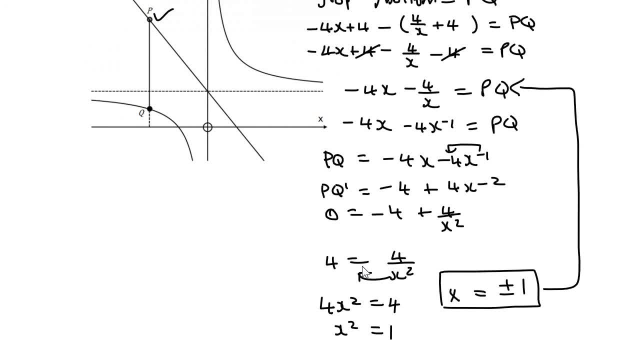 of pq over here, for example. and so if x is 1, then pq is going to be minus 4 times by 1, minus 4 over 1, and that's going to give us minus 8.. You can't have a length that is negative, so that's not even applicable. And then if x is 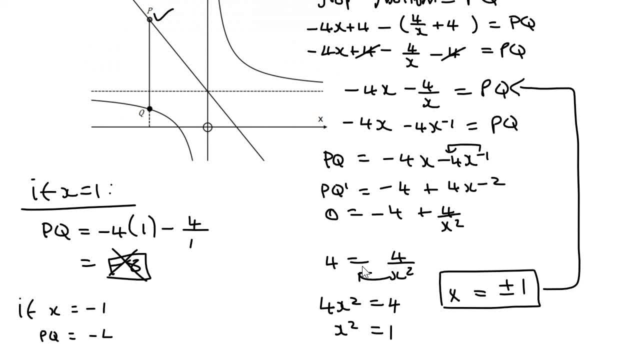 minus 1,, pq is going to be minus 4 times by minus 1,, minus 4 over minus 1, and that's going to give us positive 8, and that's applicable. So that is the answer.